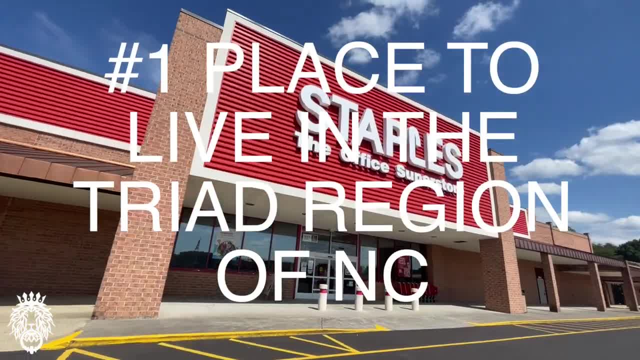 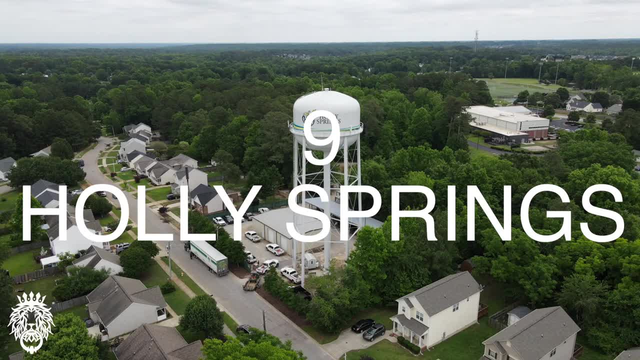 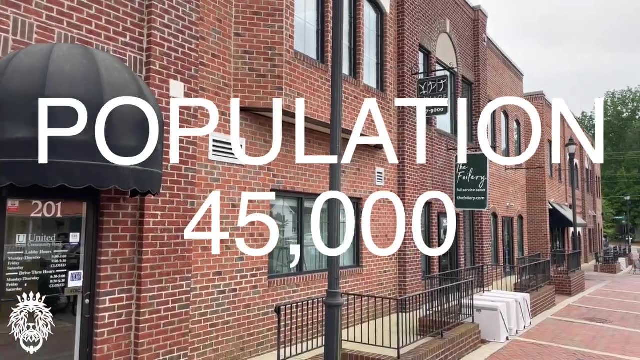 Nichecom rates Clemens the number one place to live in the triad region of North Carolina. Next up in the number nine slot we have Holly Springs, North Carolina. Holly Springs is a community very close to Raleigh with a population of around 45,000 people. Holly Springs is about 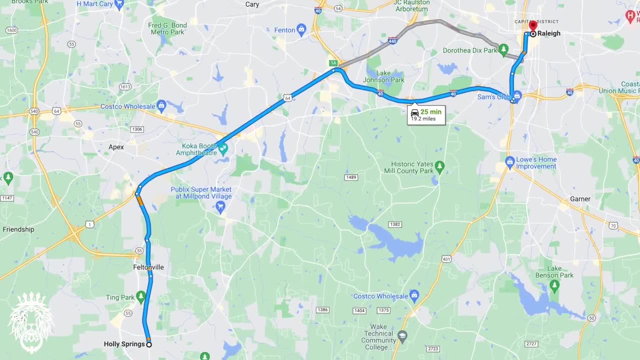 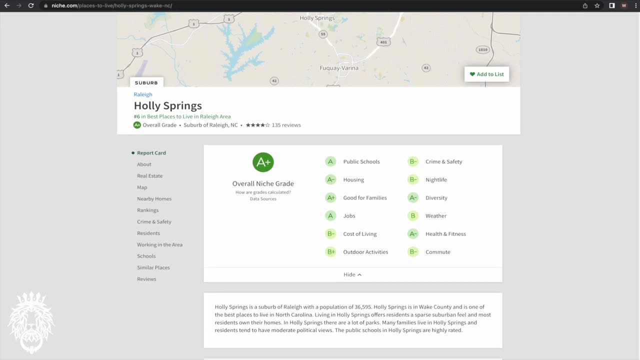 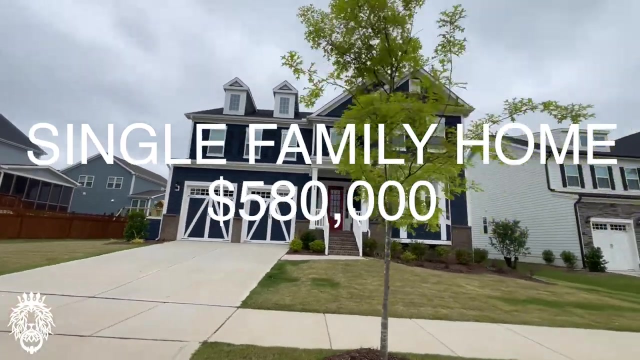 25 to 30 minutes from downtown Raleigh and Nichecom gives the town an A+. an overall rating of A+. Public schools in Holly Springs get an A with Nichecom and housing gets an A- Median home price currently in Holly Springs comes in at $580,000.. Median household. 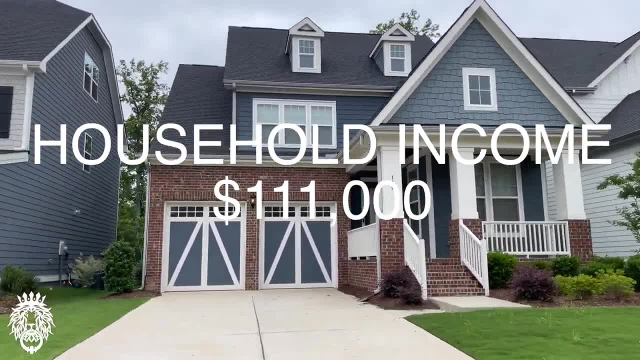 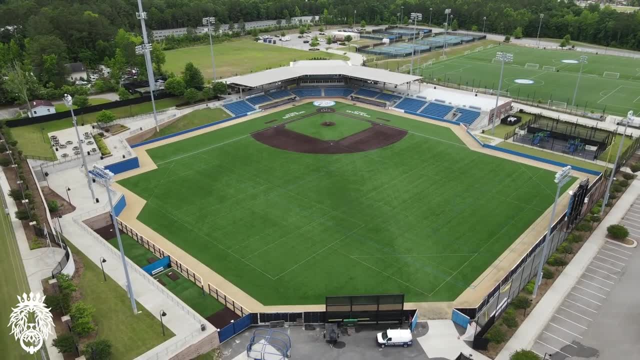 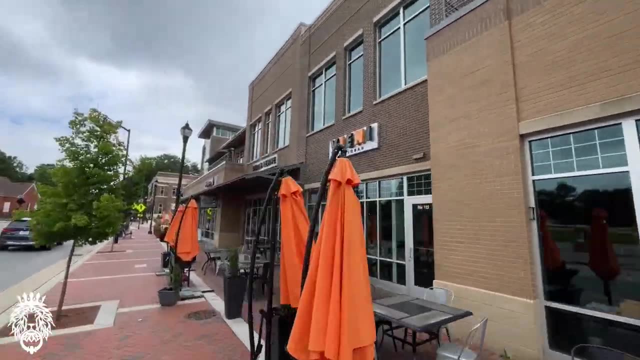 income comes in at $111,000.. So we've done a video about Holly Springs by itself recently. Recommend you guys check that out. It is a really really nice town but it's pretty much what you would call a new suburb in that it was really really small just a few years ago and it's really grown rapidly. Lots of people have moved to Holly Springs because of the quality of life and the location, the proximity to Cary and Raleigh, So it's really, really cool. but it suffers in that it doesn't really have an amazing downtown. that kind of grew up over the years and years and 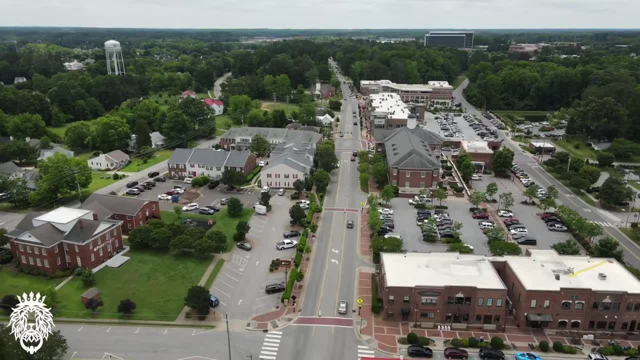 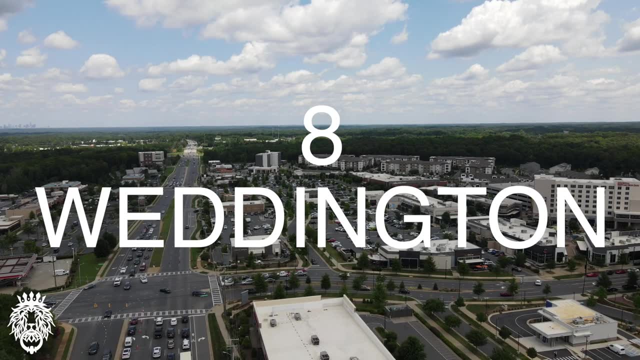 years. It's pretty much a new downtown, but people that live there absolutely love it and that's why it ranks so high on this list. Next up in the number eight slot we have Weddington, North Carolina, And having lived in North Carolina my entire life, 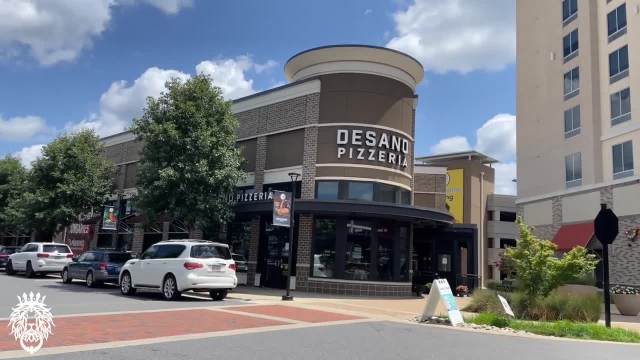 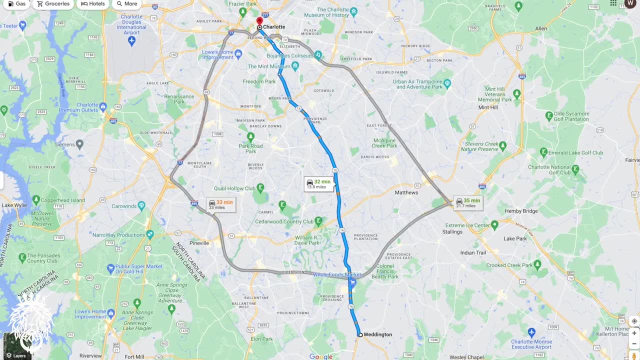 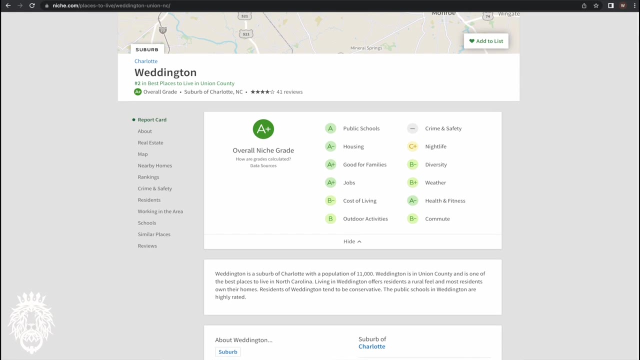 I have never heard of Weddington. It's a suburb outside of Charlotte, has a population of only 14,000 people and it is about 30 minutes from downtown Charlotte. Weddington gets an overall rating on Nichecom of A+. Public schools get an A and housing gets an A- on Nichecom. 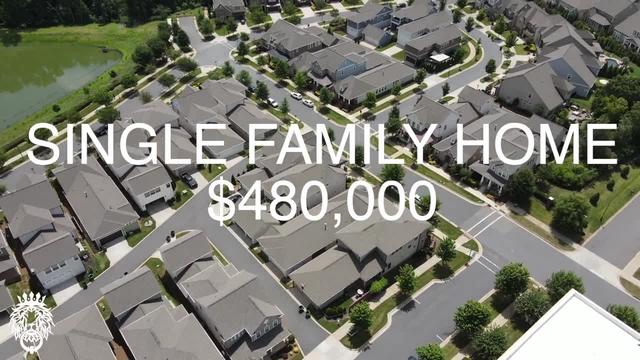 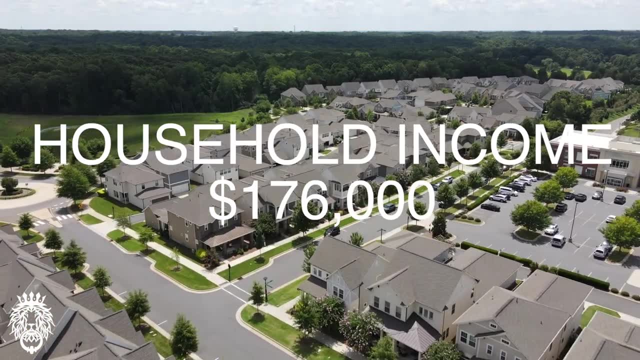 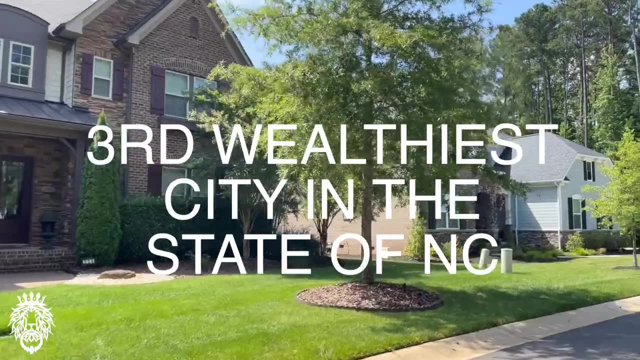 Median home price for a home in Weddington right now is in the range of about $480,000. And median income comes in at $176,000.. So Weddington is a small town to the southeast of Charlotte and it comes in as the third wealthiest city in the. 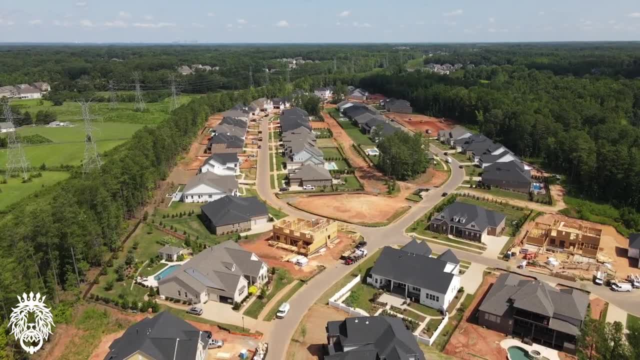 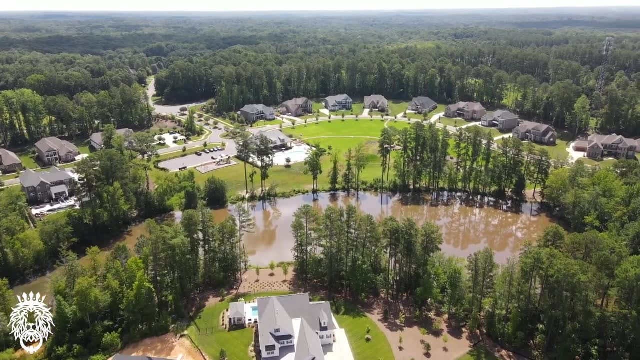 entire state, Shocked that I've never heard of Weddington before, but just looking at some of the real estate in this town, it's really, really a nice town, great location. Apparently, according to Niche, the schools are fantastic And it comes in as the number one, number two, number three. number three, number four, number five, number six, number seven, number eight, number nine, number nine, number ten, number eleven, number, eleven number, eleven, number twelve, number twelve, number twenty, number, twenty-two number, twenty-two number, twenty-two, number, twenty-three number. 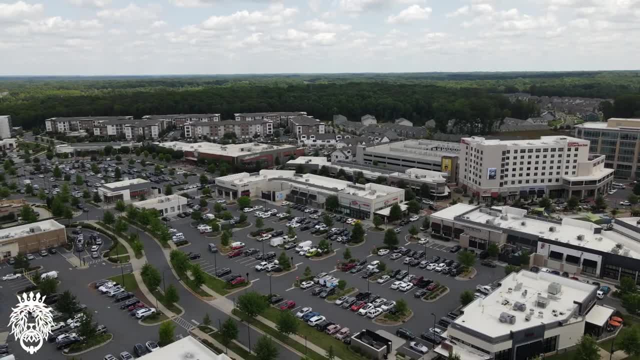 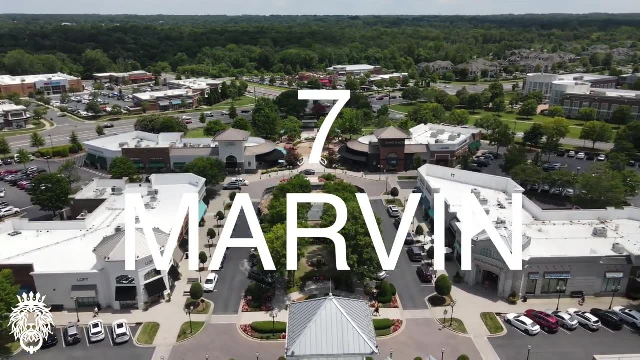 twenty-three, number twenty-two and number twenty-three, So Weddington is the number two best place to live in Union County, according to Niche. Next up in this number seven slot is another town near Charlotte, Marvin, North Carolina. Marvin has a population of only 6,700. 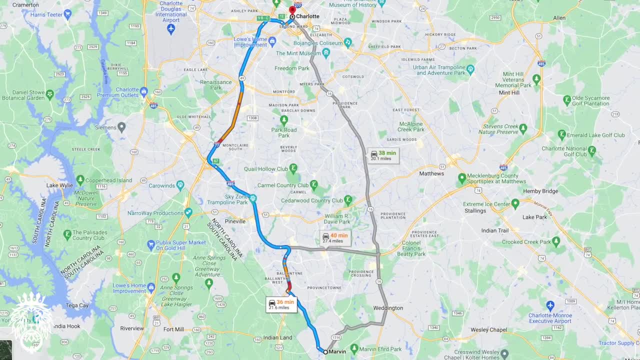 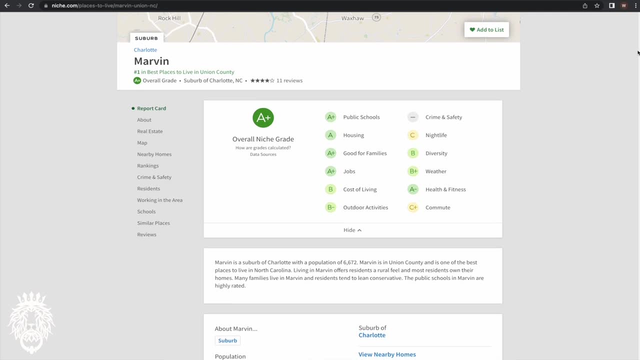 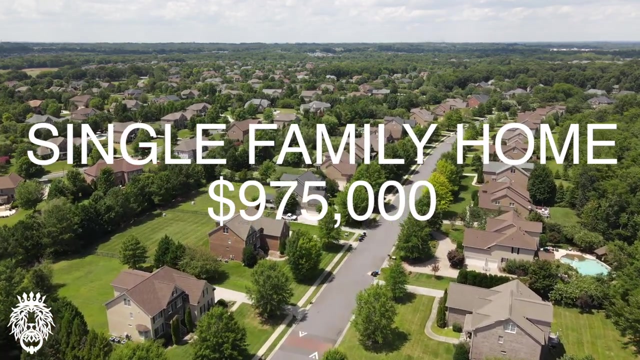 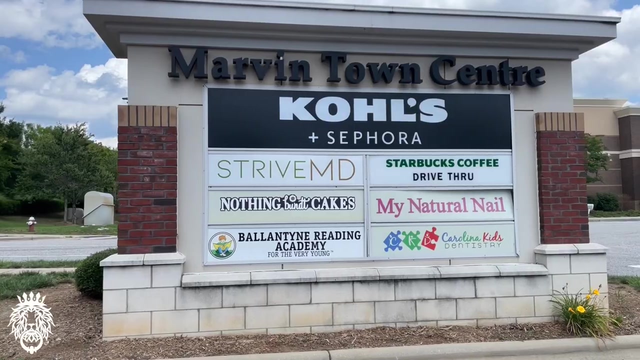 people and is about 30 minutes outside of Charlotte. Marvin gets an overall rating on Nichecom of A+, Public schools in Marvin get an A+ and housing in Marvin gets an. A Median home price in Marvin is $970,000.. With a median household income of $210,000.. Clearly Marvin has a really suburban feel. 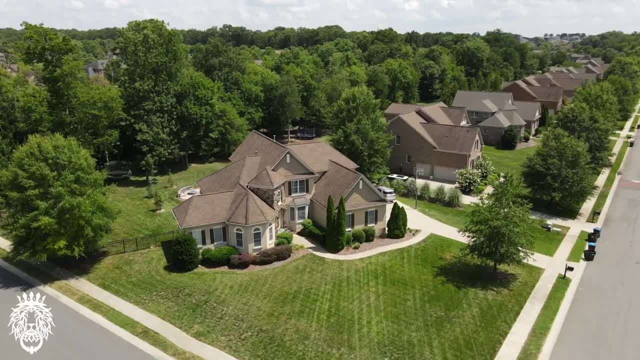 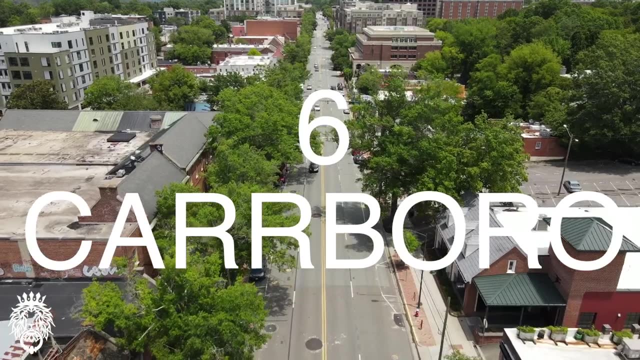 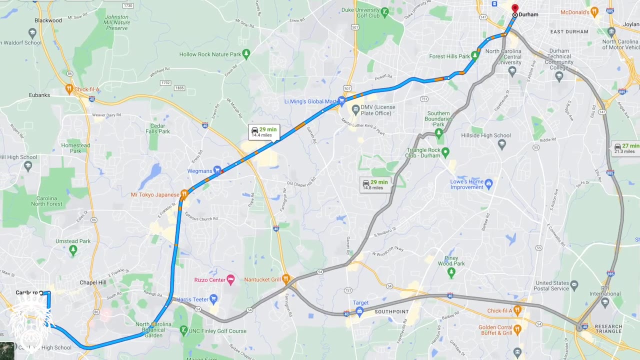 and clearly a rich suburban feel, It comes in as the number one place to live in Union County. Next up in the number six slot we have Carrboro, North Carolina. Carrboro is a suburb part of the Chapel Hill Durham metropolitan area. It's about 30 minutes away from downtown Durham and about a 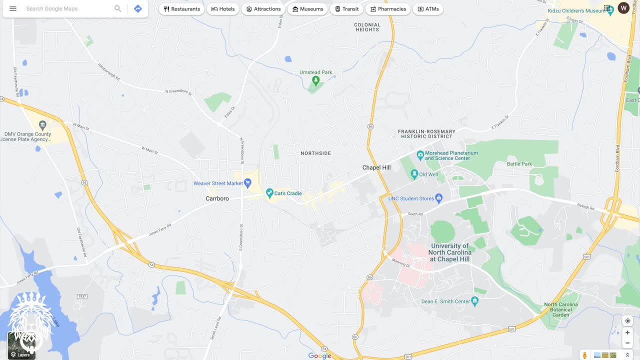 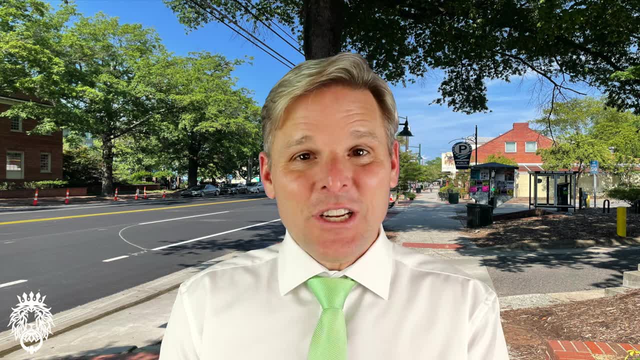 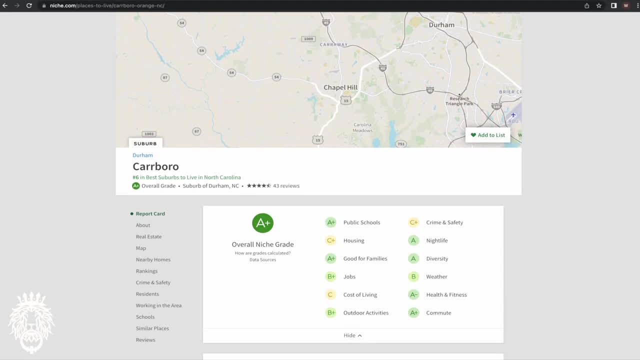 Chapel Hill-Carrboro video we just did a little while ago. they're pretty much attached to the hip. You can't tell when you've left Carrboro and headed into Chapel Hill and vice versa. Carrboro gets an overall rating on Nichecom of A+, housing in Carrboro gets a C+ and public. schools get an A+ on Nichecom. The median home price for a home in Carrboro currently stands at around $441,000. And the median household income it's coming in at $68,000.. So the best way to describe Carrboro is it sort of has an urban. 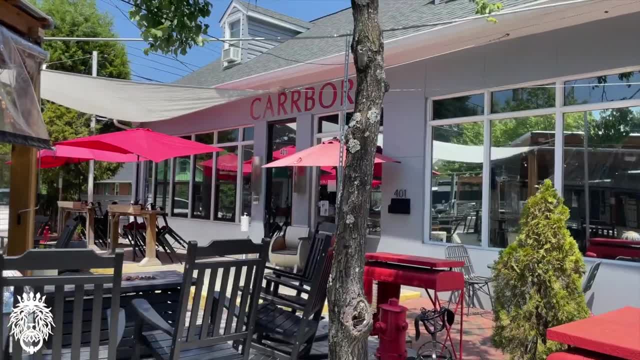 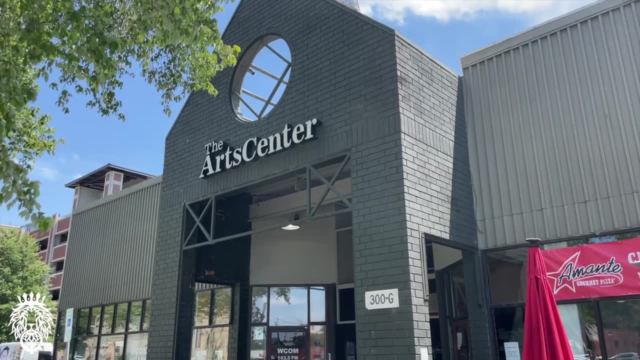 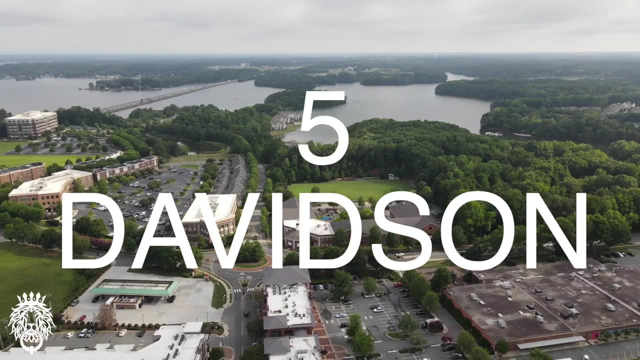 suburban kind of mix about it, Lots of restaurants and shops, sort of the smaller sister to Chapel Hill, Really really kind of funky and neat place to go visit, neat place to live. Next up in the number five slot is Davidson, North Carolina. Davidson is another suburb. of Charlotte, with a population of around 13,000 people. Davidson is about 30 minutes from downtown Charlotte and is most well known for being the home of Davidson College, which is a very, very prominent, very difficult to get into small liberal arts college, Davidson. 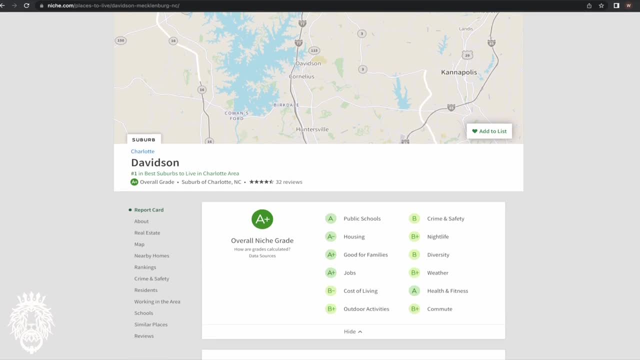 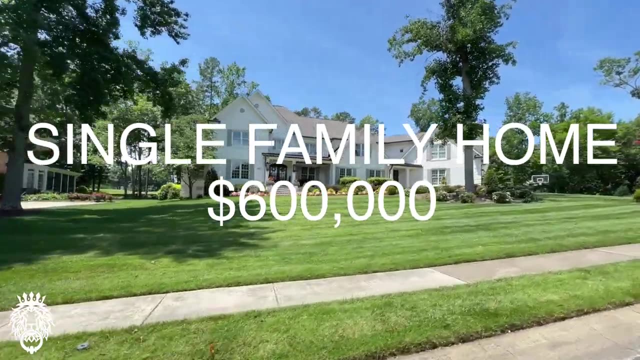 gets an overall rating on Nichecom of A+, housing gets a rating of A+ and public schools gets an A. Median home price currently sits at $600,000 in Davidson, North Carolina, while the median household income comes in at $131,000. 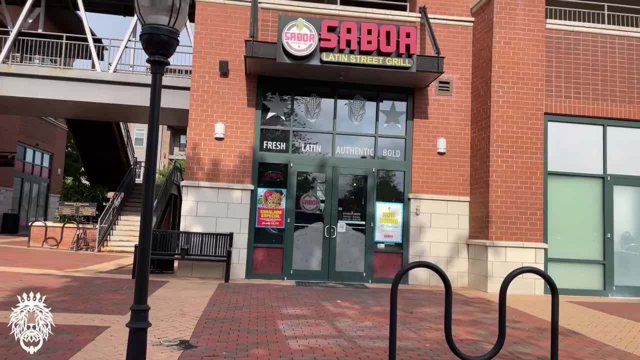 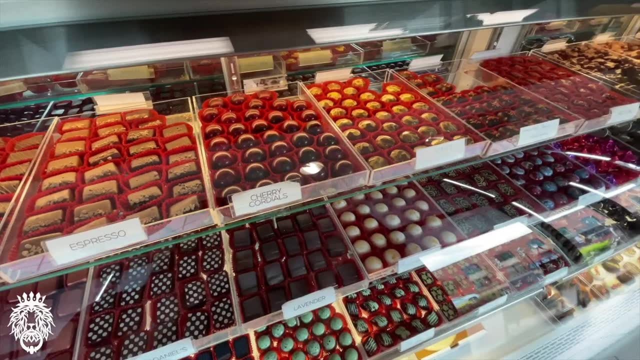 So Davidson has a very college suburban feel: lots of shops, coffee shops, restaurants, that sort of thing, Again completely dominated by Davidson College. but because it's so close to Charlotte, lots of people live in Davidson and work in Charlotte Also, according to Nichecom, Davidson is ranked the number one best suburb around Charlotte, Next up in the number four slot. another Raleigh suburb, Apex. Apex, again close to Raleigh, North Carolina, with a population of about 30,000 people. Apex, again close to Raleigh, North Carolina. with a population of about 30,000 people. Apex, again close to Raleigh, North Carolina, with a population of around 63,000 residents. It's about 20 minutes to downtown Raleigh and Nichecom gives Apex an overall rating of A+. Public schools in Apex get an A and housing in Apex gets an A. on. 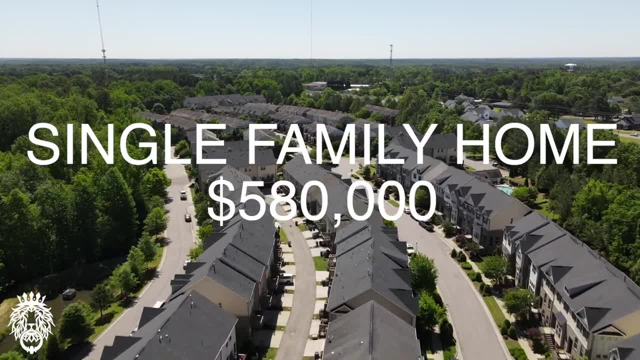 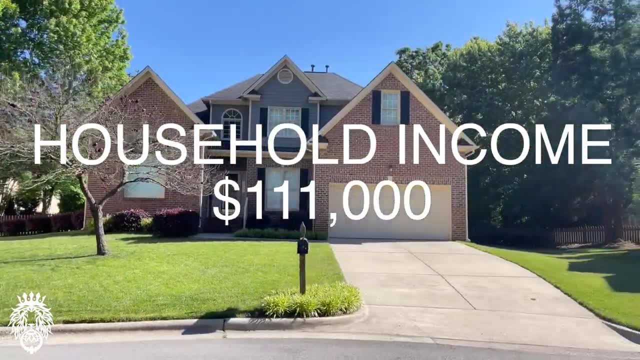 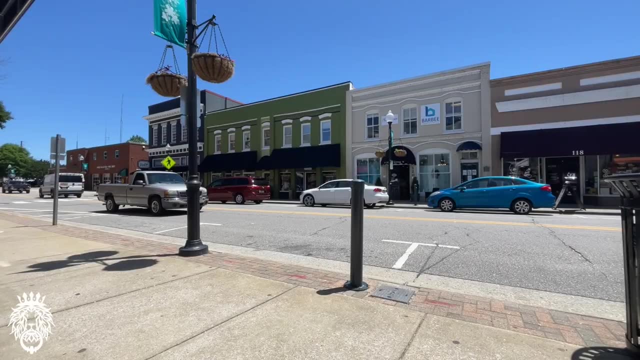 Nichecom as well. Median home price is currently sitting at around $580,000. The median household income in Apex, North Carolina, is sitting around $111,000.. So, as we've said before in the Apex video, it's a very suburban town, very, very, very close to Cary. Lots of people live in. 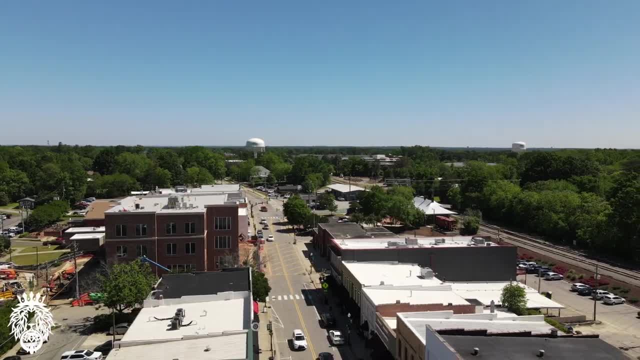 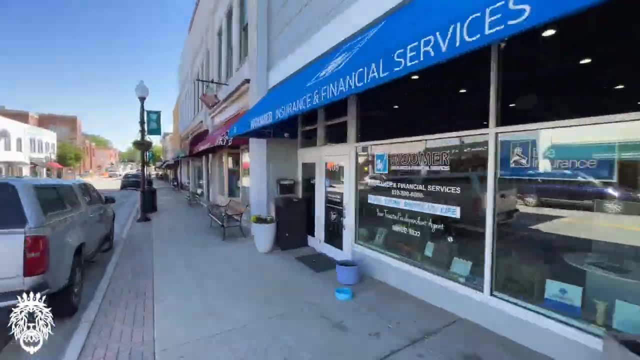 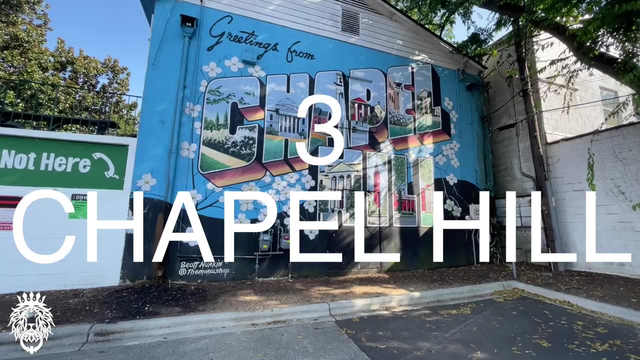 Apex work in Cary or work in Research Triangle Park or maybe work in downtown Raleigh. Lots of great shopping, lots of really cool restaurants. Apex wings And Nichecom ranks Apex the number three best place to raise a family in North Carolina. Next up in the number three slot is Chapel Hill, North Carolina. And you guessed it, Chapel Hill is part of the Chapel Hill- Durham metropolitan area. Chapel Hill has a current population of around 63,000 residents. Chapel Hill is about 38 minutes from downtown Raleigh and about 25 minutes to downtown Durham. 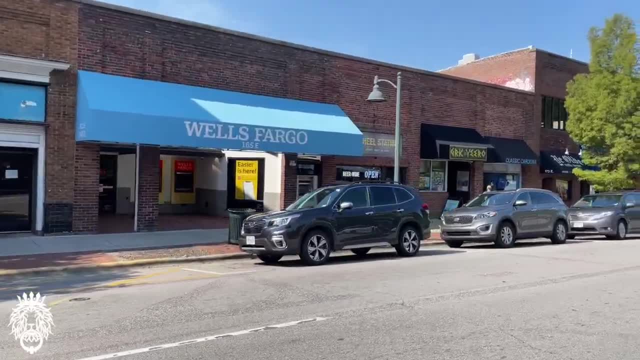 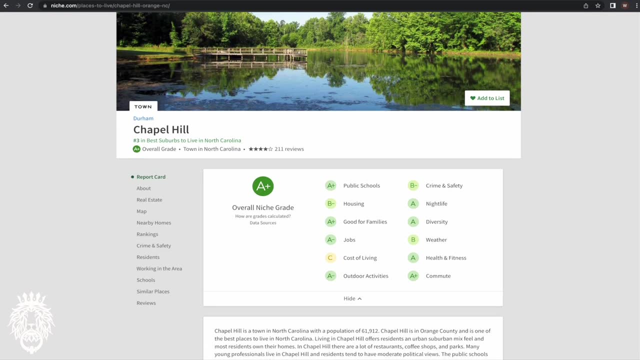 Although you're very, very close, like 10 minutes, 15 minutes from the streets at South Point part of Durham, Chapel Hill gets an overall rating on Nichecom of A+. Public schools in Chapel Hill get an A+ as well and housing gets a B- Median home price. 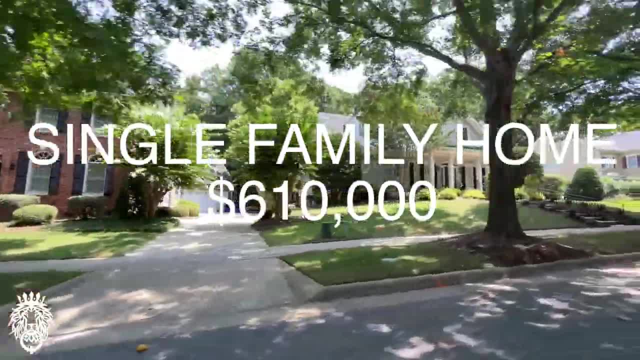 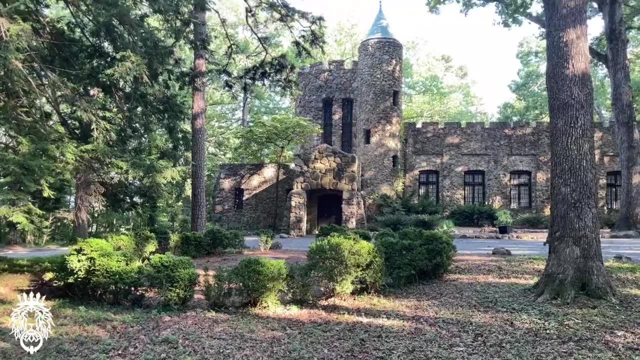 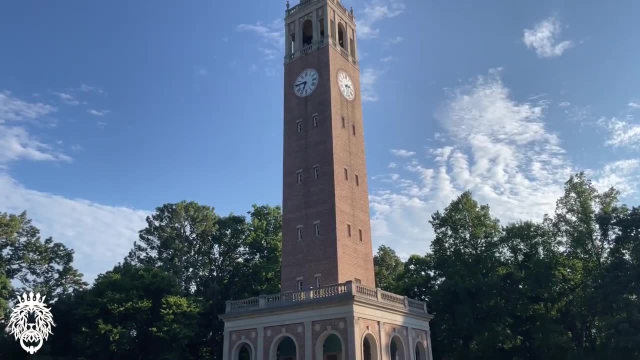 in Chapel Hill currently is $610,000.. Median household income in Chapel Hill is $123,000. And, of course, as we said in our Chapel Hill video, Chapel Hill, the town is dominated by the University of North Carolina. at Chapel Hill. It is the quintessential college town, very small. village vibe to it, although it is growing and growing, and growing. in the last few years, Those of us that went to UNC can barely recognize the town anymore. There's been so much growth going on. It's a place to live, as evidenced by how high it ranks on this list. Definitely worth your time to. go check out Chapel Hill- Great staycation, vacation kind of thing if you want to do that, or maybe somewhere you want to move and have a permanent vacation. Next up in the number two slot is Cary, North Carolina. Cary is a suburb of Raleigh and is in fact probably the quintessential suburb of Raleigh. Currently, 183,000 people live in Cary And, again, as I said, Cary is probably the quintessential suburb of Raleigh because it's so terribly close to Raleigh: Only 18 minutes to get from Cary to downtown Raleigh. 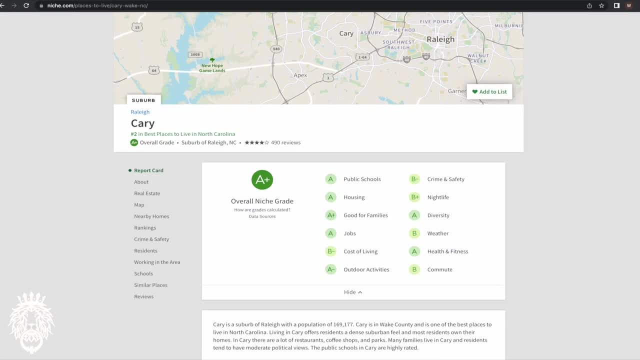 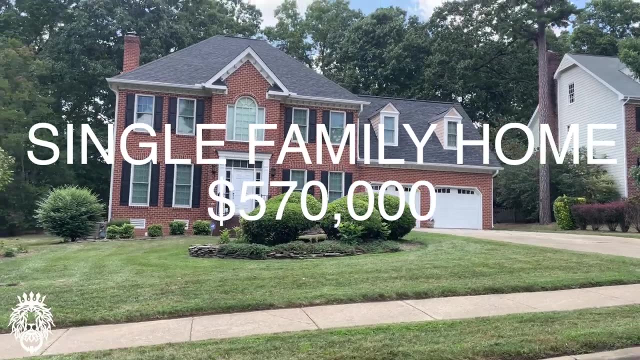 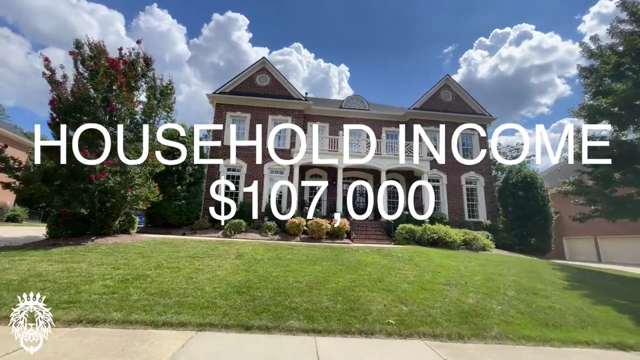 Nichecom gives Cary an overall rating of A+. Public schools in Cary get an A and housing in Cary also gets an A. with Nichecom, Median home price is coming in at $570,000 currently and median household income is coming in at $107,000 currently. Cary has a very suburban. city. It is again a place that a lot of people live, that work in downtown Raleigh- Research Triangle Park- And in fact Cary, owes its growth to the birth and the growth that's happened in the Research Triangle Park area And because it's really in the middle of the triangle, people can live in Cary and work just about anywhere in the area that they choose to work. Next up in the number one slot we have Morrisville, North Carolina. Morrisville is another suburb of Raleigh, 20,000 people currently calling Morrisville home. Morrisville is about 20 minutes from downtown.